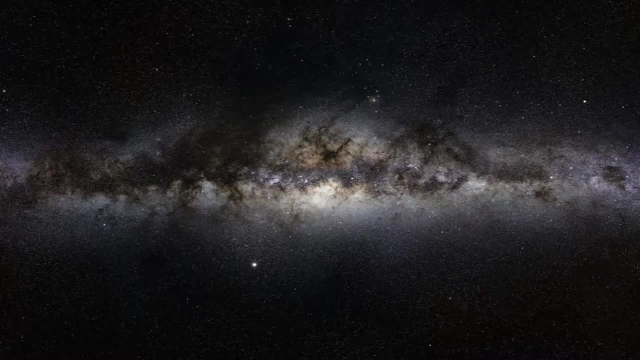 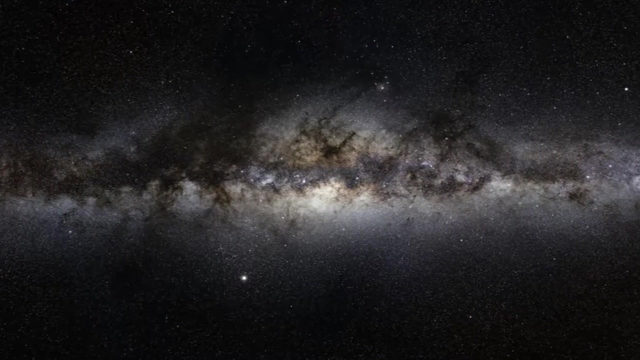 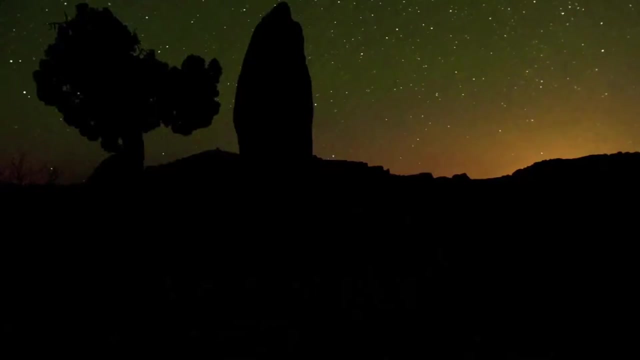 the strange illuminated clouds in the sky. What does it say? The feature that defined the night sky for most of humanity's existence can no longer be seen or even recognized by a large amount of people. Not being able to view the stars may seem trivial, but it has global effects. The sun is the 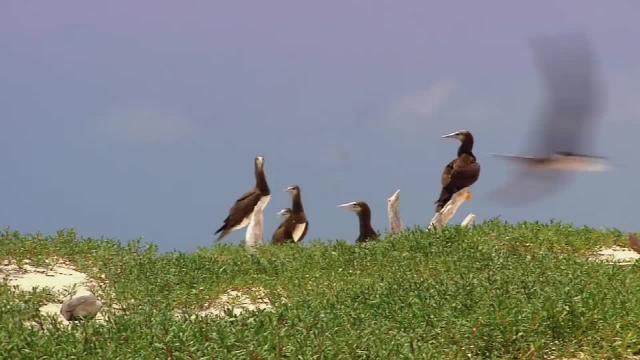 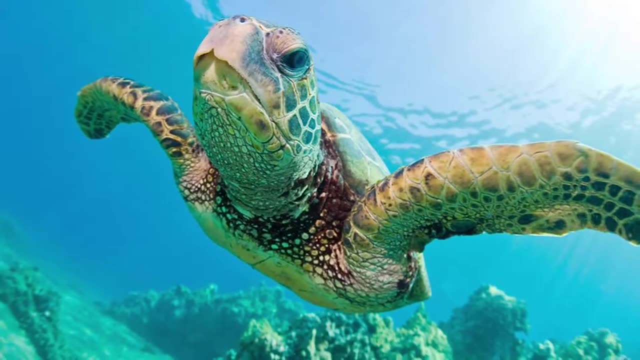 center of our universe, but life continues when the sun goes down. The sun is the center of our life. Animals, birds and reptiles alike all rely on 24-hour days. Animals eat and migrate at night. Sea turtles lay their eggs on beaches at night, But now that the night is turning to day, these 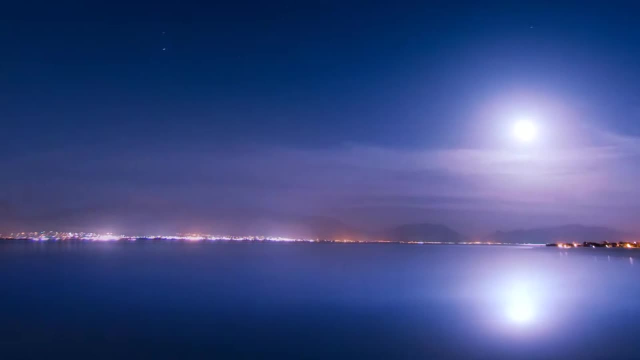 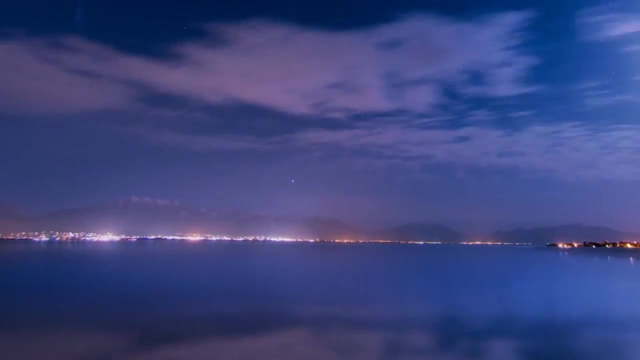 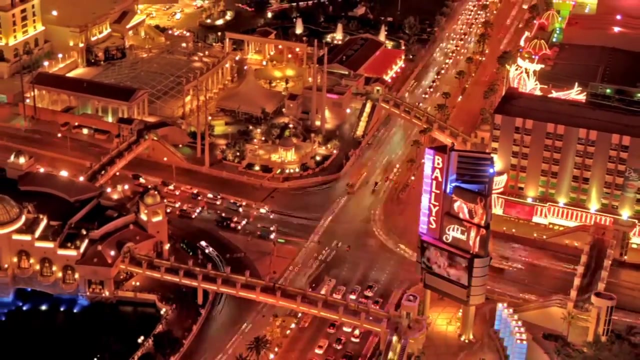 creatures can no longer tell when is night and when is day. These delicate ecosystems that rely on the natural balance of the ecosystems are becoming more and more erratic. Light during the night can also affect the environment. The sun is the center of our life. The sun can also affect humans. Glare from street lights can cause disability, glare that 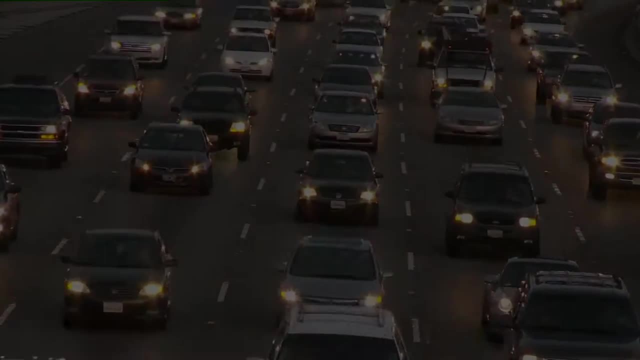 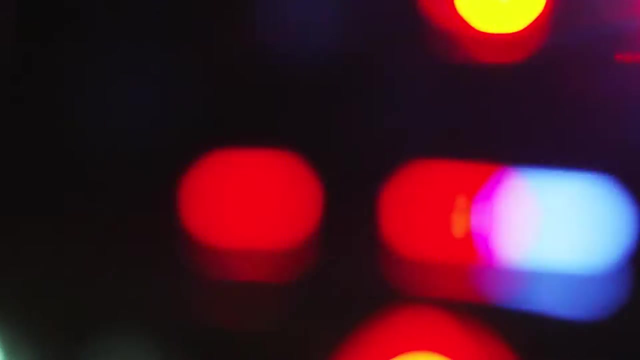 causes drivers to see only the light, casting everything else into invisibility. Criminals can also use light at night to hide. By standing behind a light, the person becomes invisible, allowing for an increase in crime. The biggest problem for human health, however, is human. 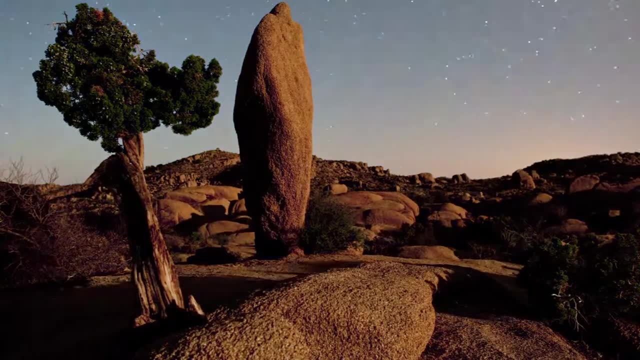 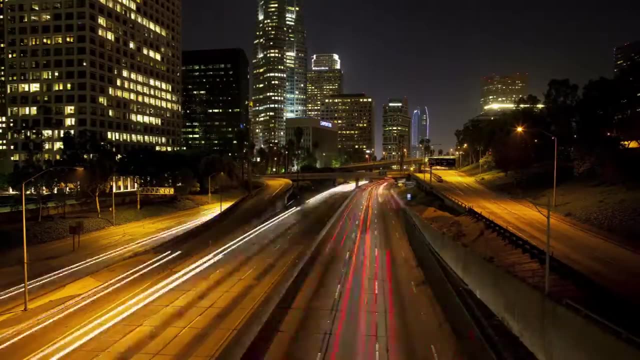 cycles. Human circadian rhythm is a human's natural 24-hour cycle. Now, with light pollution, the cycle is being impeached. Instead of rising with the sun and going to bed with the sun, people can wake up when they want to. The sun is the center of our life. The sun is the center of our 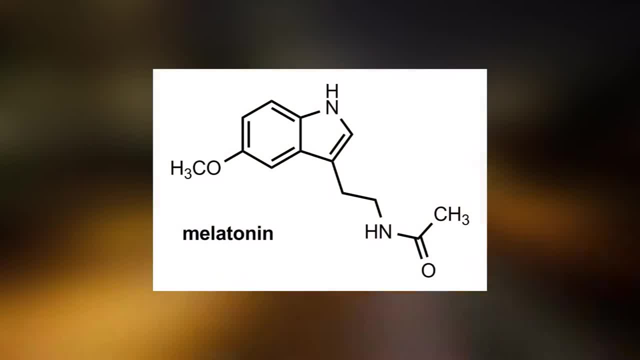 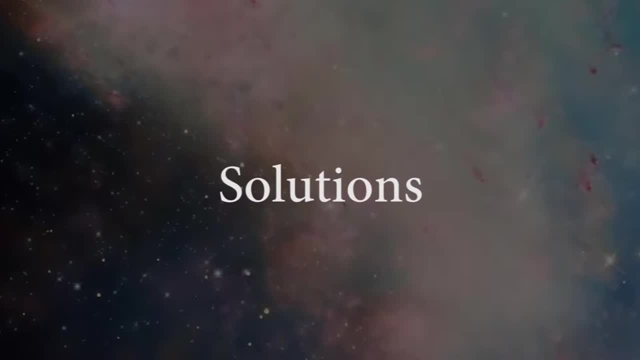 being Because we're the source of life. light is patient. Light can also lower the levels the body requests to regulate its hormones. Light also senses melatonin, infinitary Presidential compounds that regulate hormones. Light may release acted drawing sessionsbank easy to read the STDs, despite which it is difficult to release the sends Private. 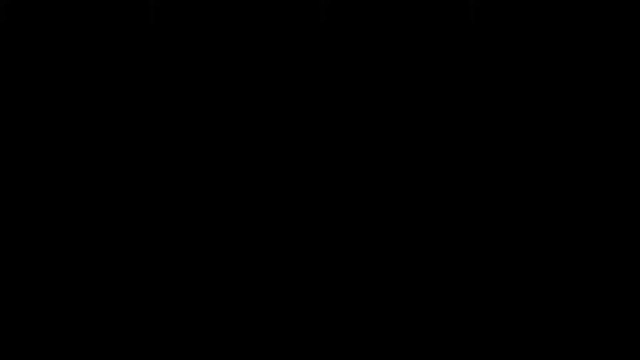 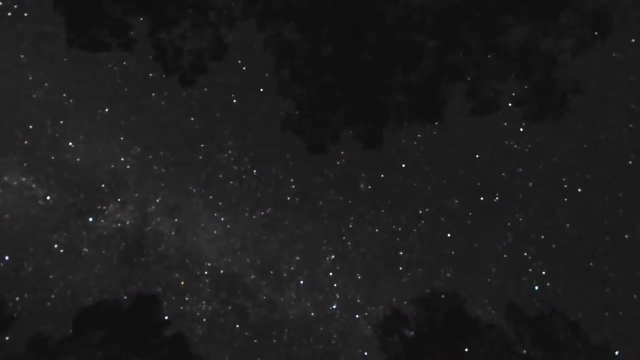 Penetrating Antibody for Outerинки Iron. Light pollution is often a daunting task to tackle, as it may seem bigger than any one person to fix or even begin to stop Light pollution is, and if everyone does their part, then someday soon we will be able to glance up at the night sky and marvel at its beauty. 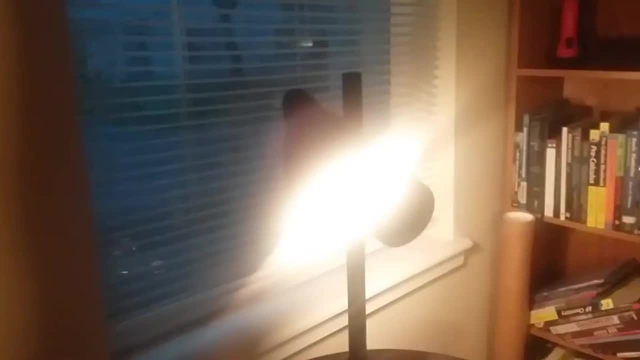 So how do you fix it? Just normal, brings your light back into the light of a new dawn To start with, where we are seeing the stars. gonna do a day or two, whatever will be a. Just do a couple of easy things.